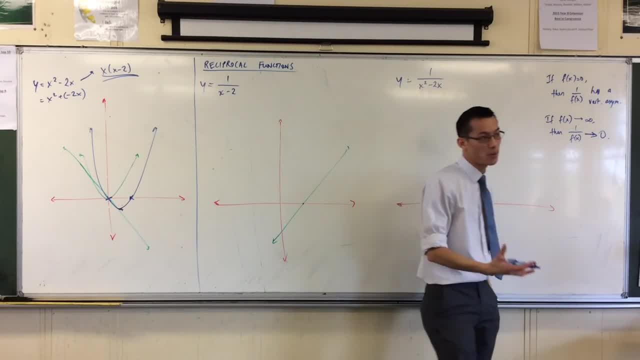 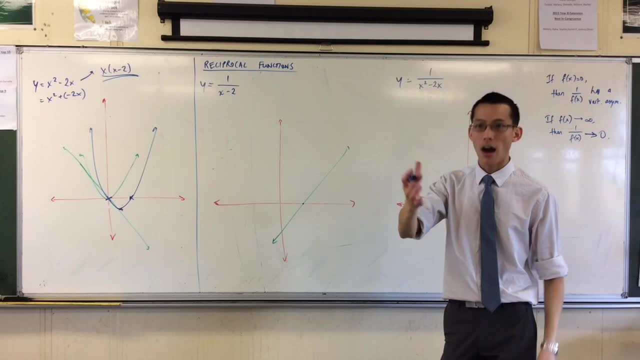 So, for example here- here's the first important point- I notice This guy here, right, The function is zero there. So when I think about its reciprocal, I ought to be expecting: well, I can't exist there, right? 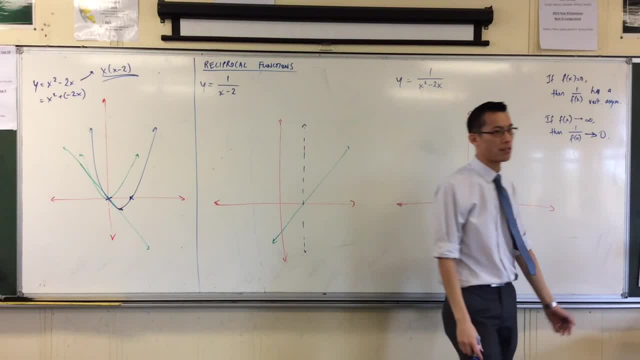 So I'm going to pop a vertical asymptote through there. Are you okay with that? Okay, Now, when you have a look over here, I'm going off to infinity right, And there's no limitation on it, okay. 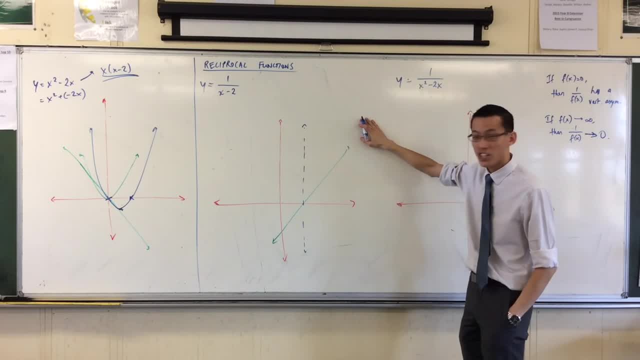 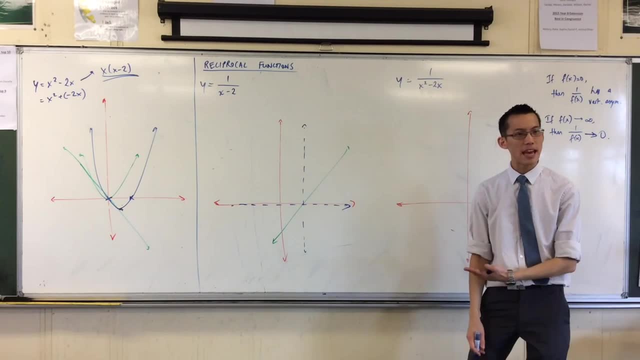 So when I take the reciprocal of something that's growing, it's going to come down to zero. Do you agree with that? So therefore, I'm doing that. Over on the left-hand side, I observe the exact same thing. 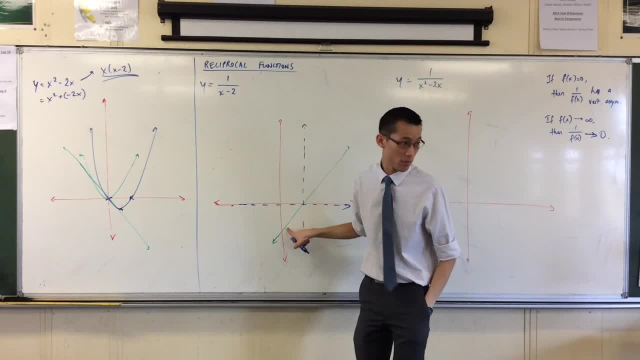 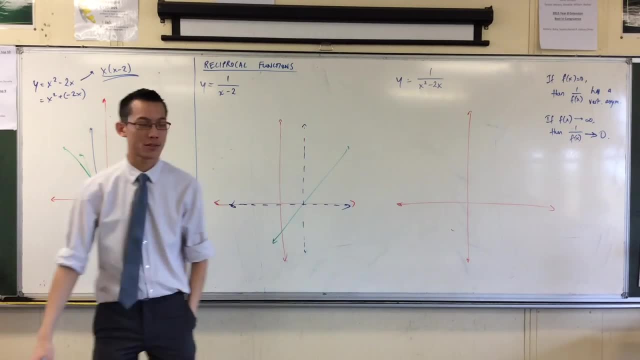 but it's going to approach from the bottom, Because it will be a small number, but it will be a small negative number. Does that make sense? So I have this asymptote horizontally on both sides. Now these are the vertical and horizontal asymptotes. 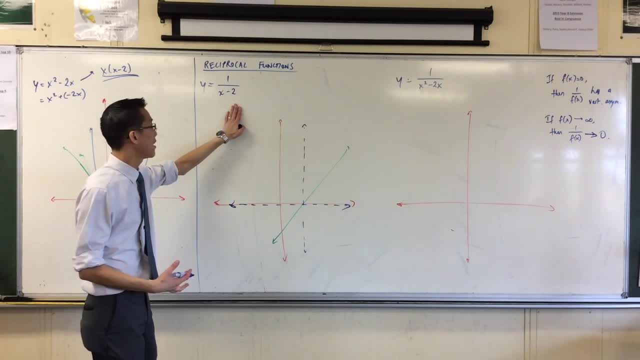 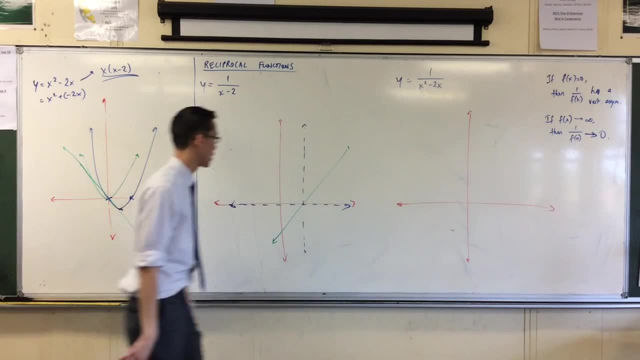 You're already familiar with because of a hyperbola right. But it's not just because it's a hyperbola right. You're using this thought process to figure out what the ordinates are doing. So now I'm going to graph the thing, right. 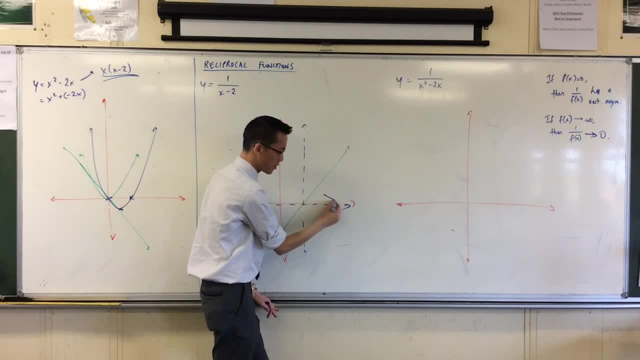 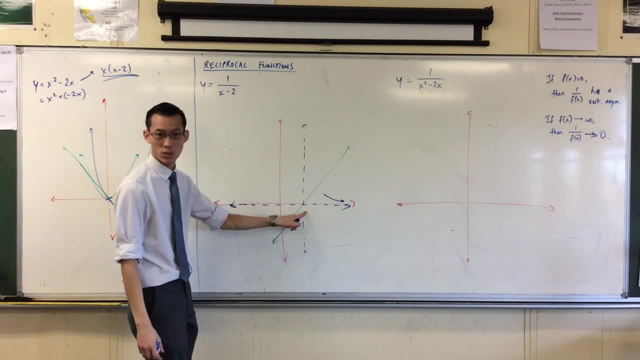 Have a look over here. I've got a really, really big positive value. So that's why I'm coming towards here. I'm dropping down like a rock, But then, as I go towards the left, towards x equals 2,. 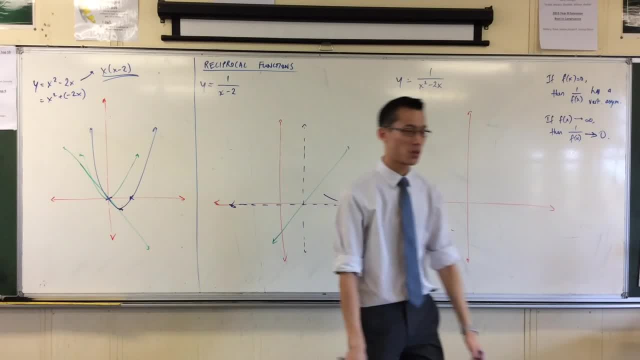 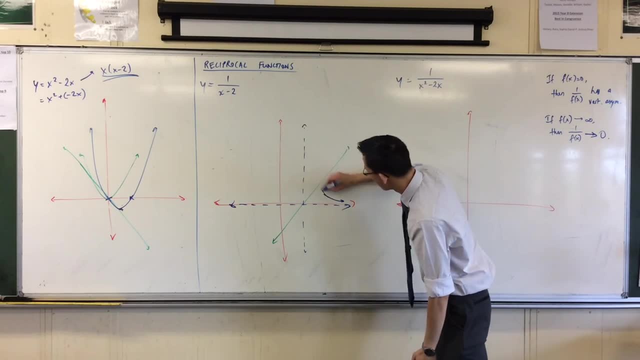 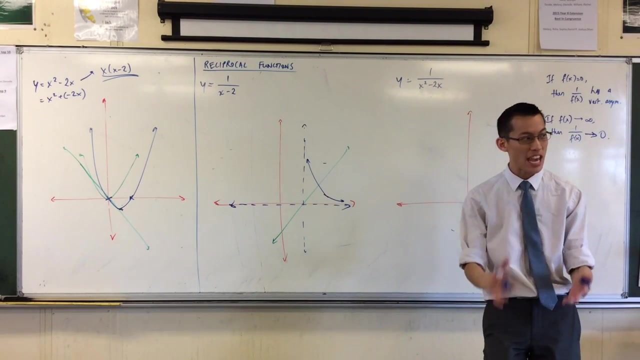 the denominator is shrinking Right, So it's going to become 1 over 0.1.. 1 over 0.001.. It's going to skyrocket. That's what it's doing Over on the left, same argument. 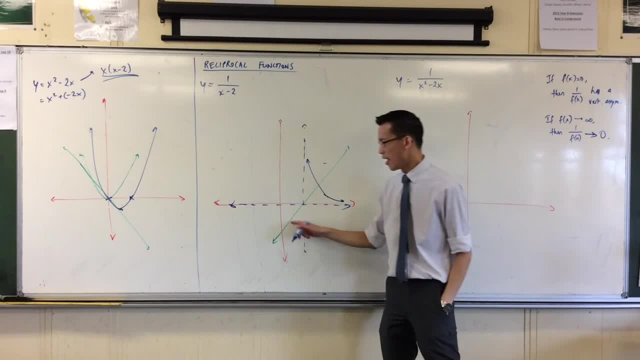 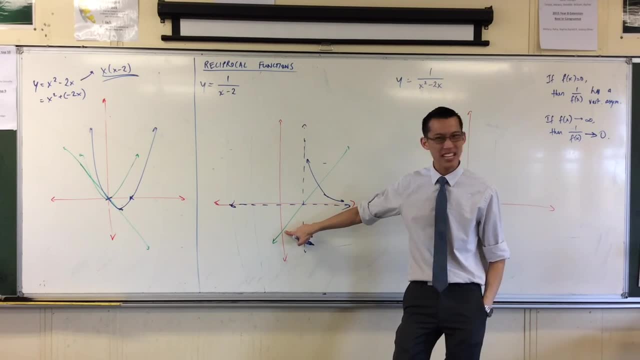 but a couple of things I can note. right, I actually have numbers here, right, I actually have numbers. So, for instance, see that, What's that intercept there? That's negative 2, right. So when I take its reciprocal, 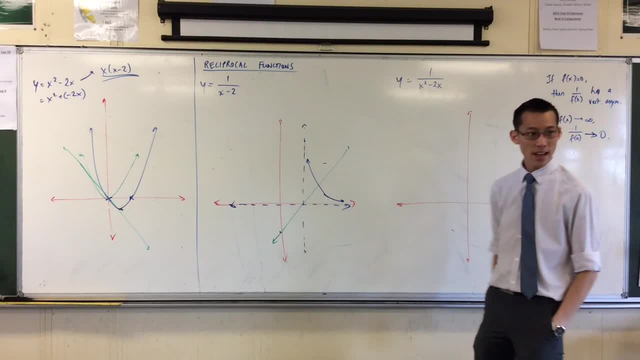 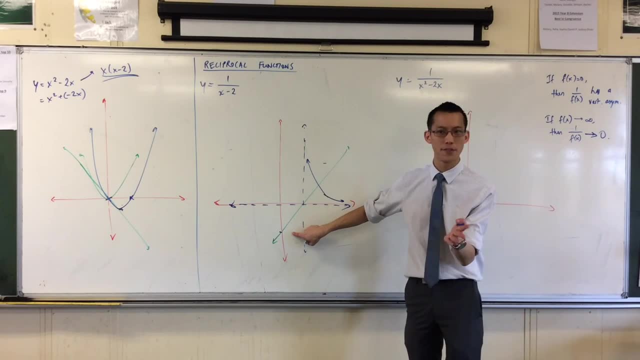 I should know what the intercept is. What's the reciprocal of negative 2? It's negative a half. right Now I actually have to know where that is, because I've said that's negative 2.. So I've logged myself into a vertical scale. 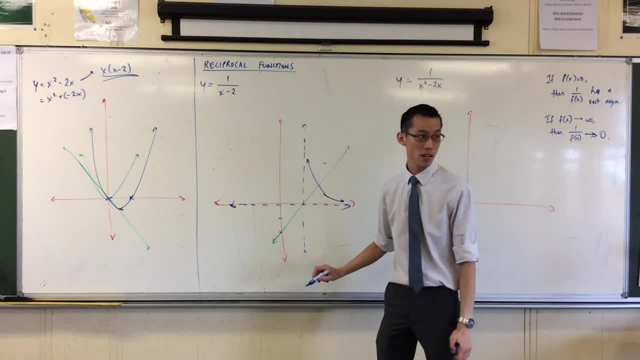 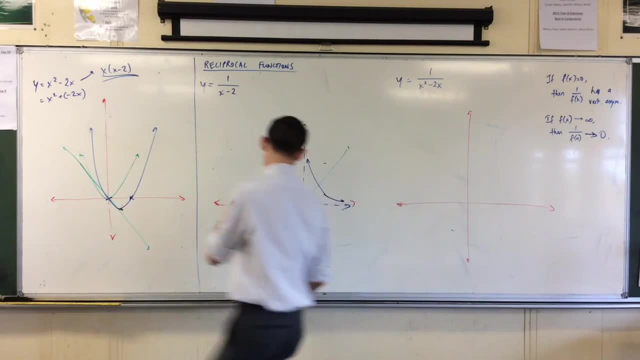 Do you notice that? So that's negative 2.. There's negative 1.. So there's negative 1 or 2.. I have to pass through there, right, Like the visual has to make a basis on that argument. 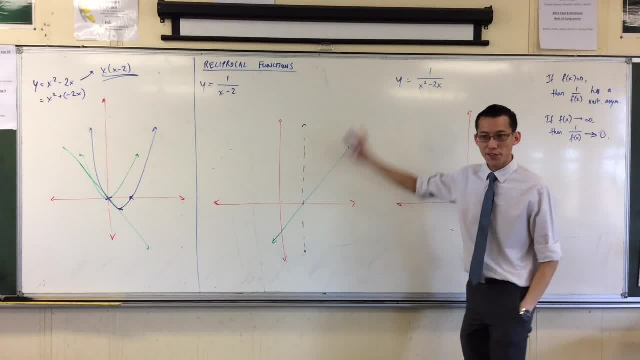 Okay, now, when you have a look over here, I'm going, I'm going off to infinity right And there's no limitation on it. okay, So when I take the reciprocal of something that's growing, it's going to come down to zero. 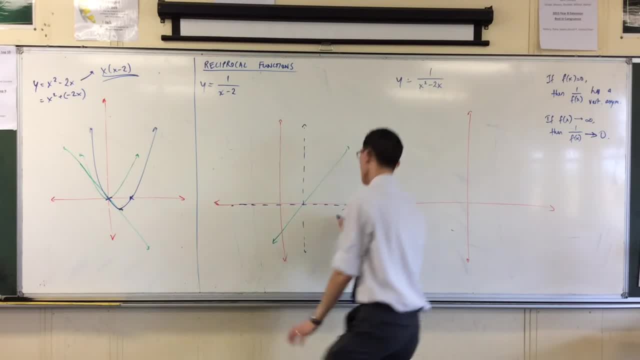 Do you agree with that? So, therefore, I'm doing that. Over on the left-hand side, I observe the exact same thing, but it's going to approach from the bottom, Because it will be a small number, but it will be a small negative number. 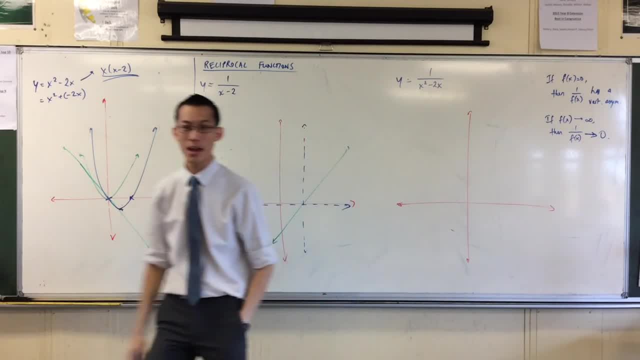 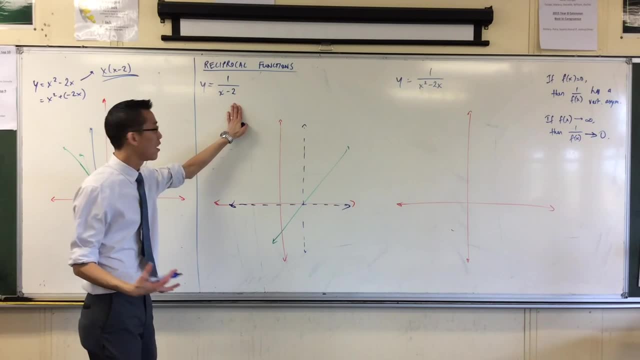 Does that make sense? So I have this asymptote horizontally on both sides. okay, Now these are the vertical and horizontal asymptotes You're already familiar with because of a hyperbola right, But it's not just because it's a hyperbola right. 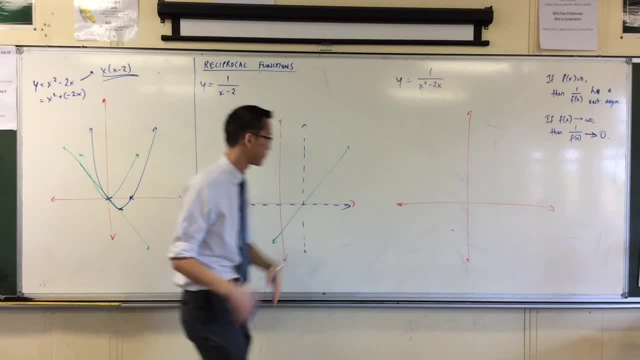 You're using this thought process to figure out what the ordinates are doing. okay, So now I'm going to graph the thing right. Have a look over here. I've got a really, really big positive value, So that's why I'm coming towards here. 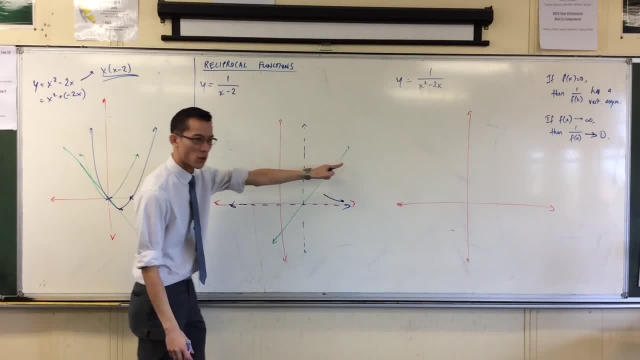 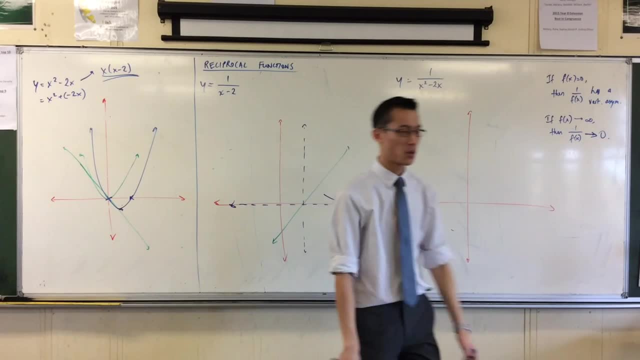 I'm dropping down like a rock, okay, But then as I go towards the left, towards x equals 2, the denominator is shrinking, It's vanishing away, right, So it's going to become 1 over 2.. 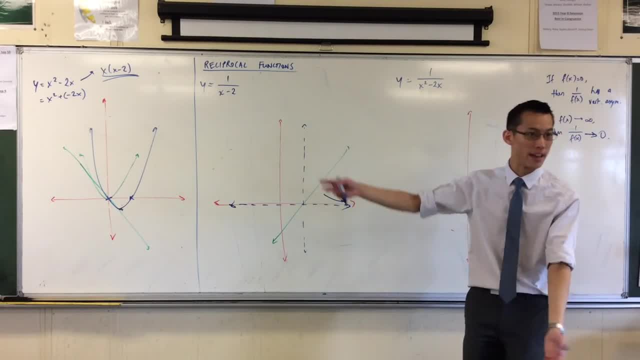 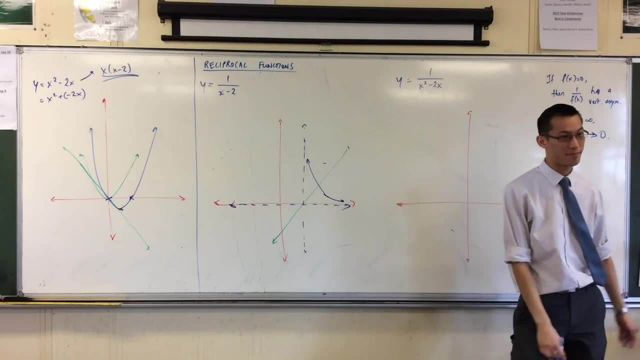 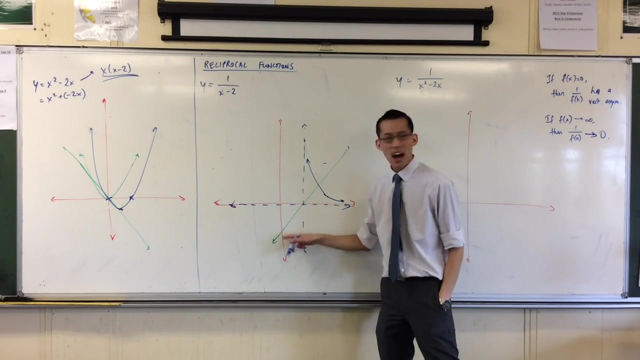 It's going to become 1 over 0.1.. 1 over 0.001.. It's going to skyrocket. That's what it's doing. Over on the left, same argument, but there are a couple of things that you don't know. 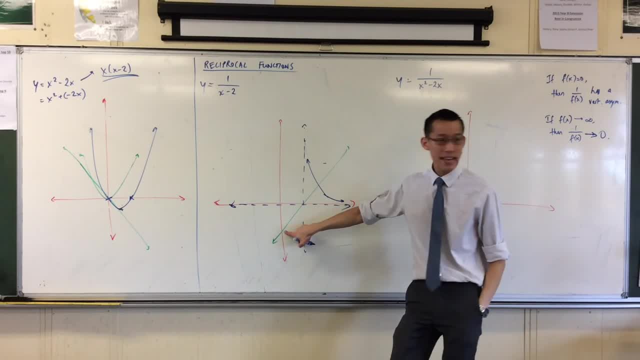 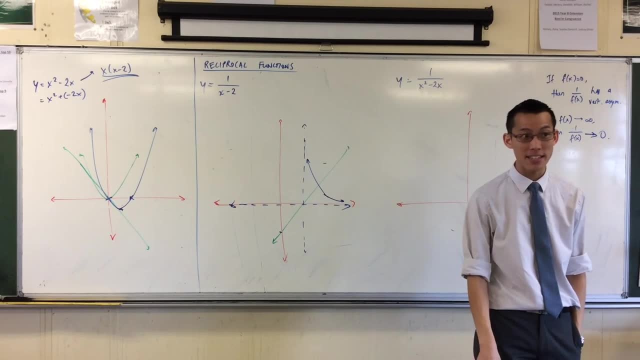 right, I actually have numbers here. Right, I actually have numbers. So, for instance, see that, What's that intercept there? That's a negative 2, right? So when I take this reciprocal, I should know what the intercept is. 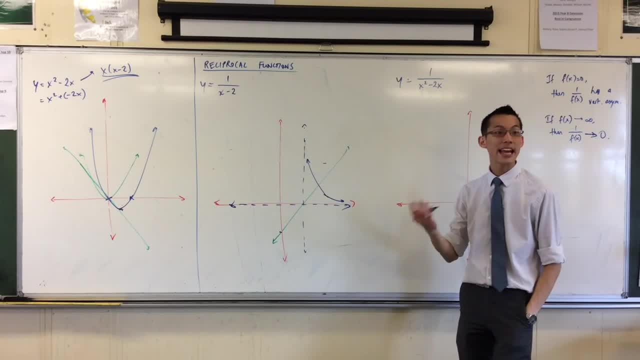 What's the reciprocal of negative 2? It's negative 1.. Negative 1., Negative 1.. Now I actually have to know where that is, because I've said that's negative 2.. So I've locked myself into a vertical scale. 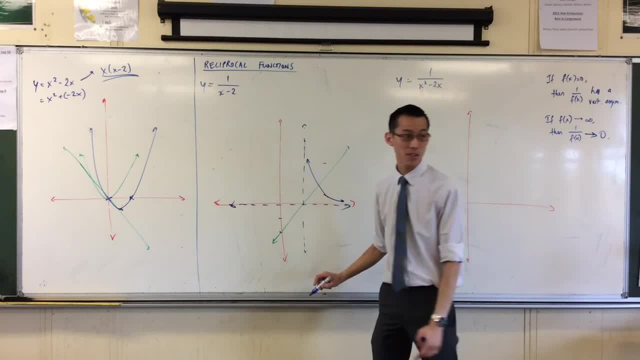 Do you notice that? So that's negative 2.. There's negative 1.. So there's negative 1 or 2.. I have to pass through there, Like the visual has to make a basis on that argument. So therefore, let's see if we can look at it there. 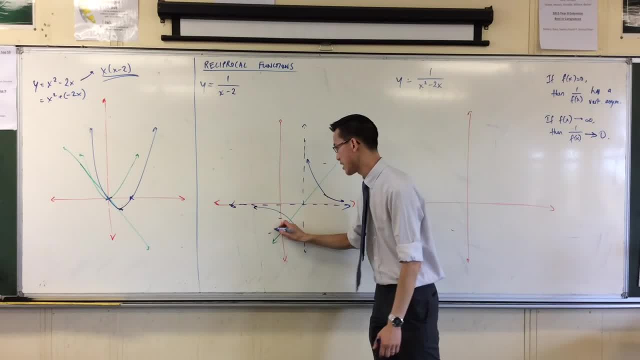 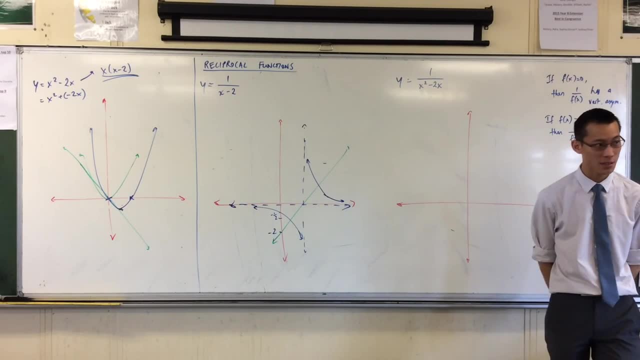 There you go, And that's actually a critical point. If I'm saying that's negative 2, then negative 1 half has to be there- It can't be somewhere else and be consistent with my vertical scale. Does that make sense? 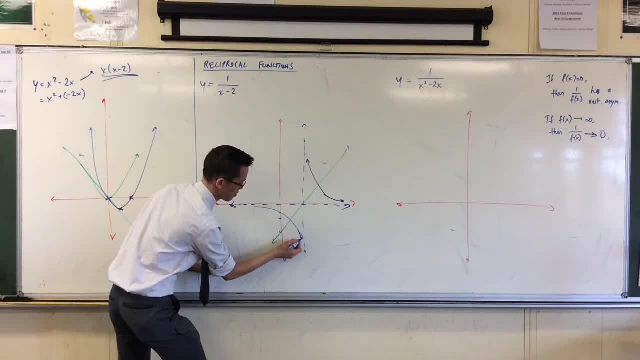 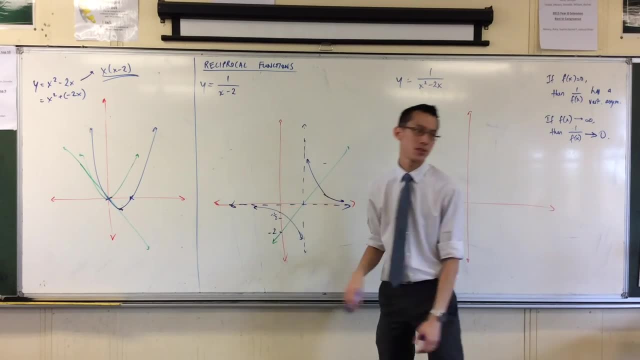 So therefore, there you go, And that's actually a critical point. If I'm saying that's negative 2, then negative a half has to be there- It can't be somewhere else- and be consistent with my vertical scale. Does that make sense? 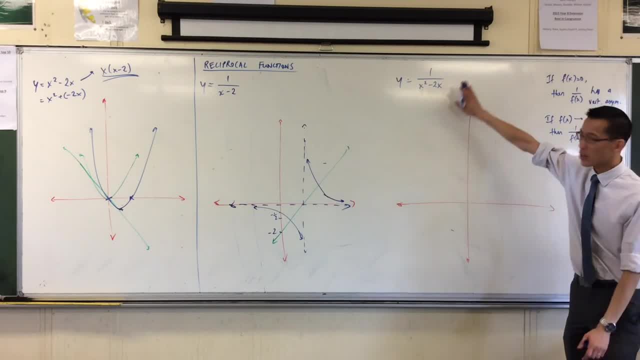 Okay, now standard hyperbola. That was a bit boring. okay, If you have a look at something like this guy, you see I've craftily chosen the graph that we just did over there, right, So let's just draw. here is our component graph. 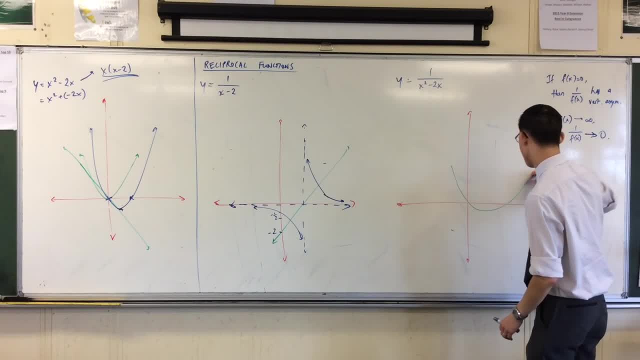 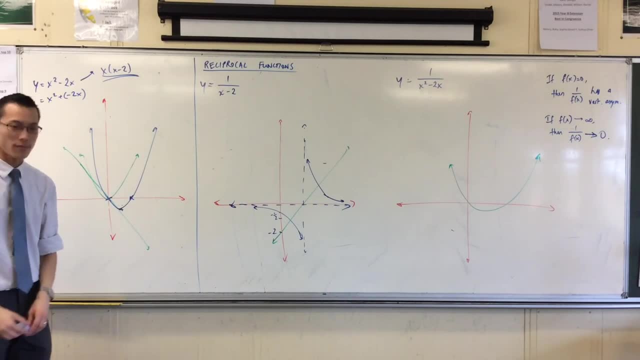 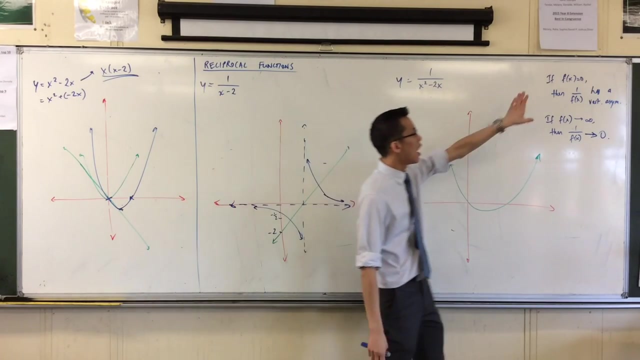 and then we can do our reciprocal Wait. so you can't? Well, you could do that, but You already know what x squared minus 2x is. okay, So now I'm going to approach this in the same way, right? 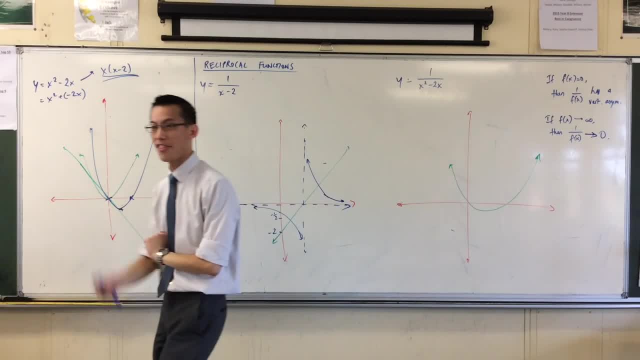 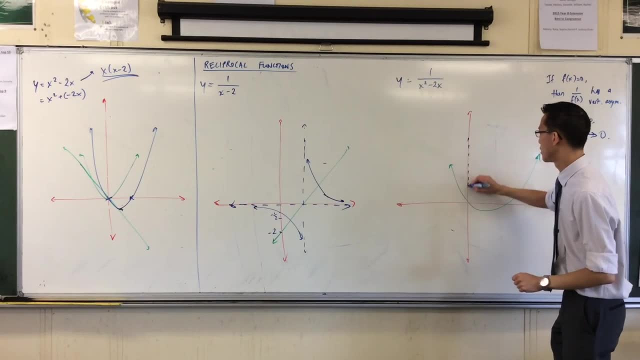 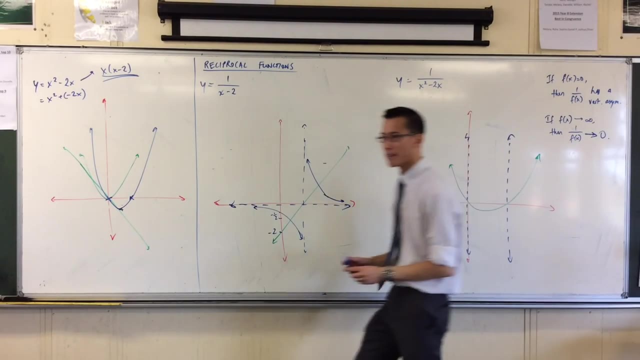 I look at the points where my function, my component function, is 0 and there are two of them, which means I've got two vertical asymptotes. right, Let's draw them in. Okay, Again, I'm going to look for my important places. 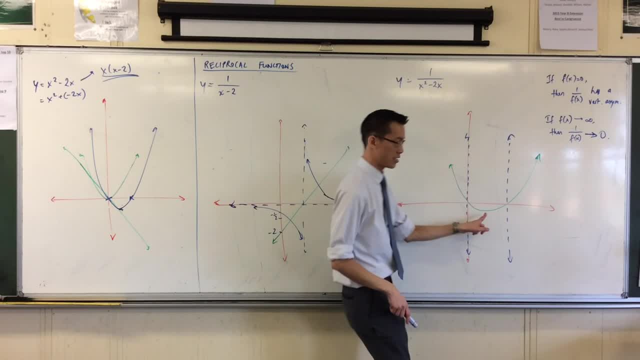 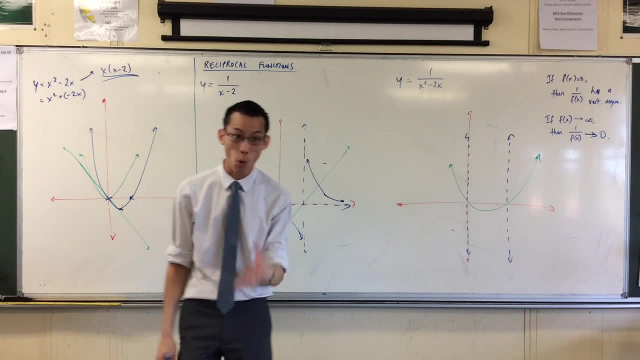 Important places. So, for instance, I actually know there's a stationary point here, right, And I can fairly easily work out its value, right? The x value is 1, so what's the y value? What's the ordinate? 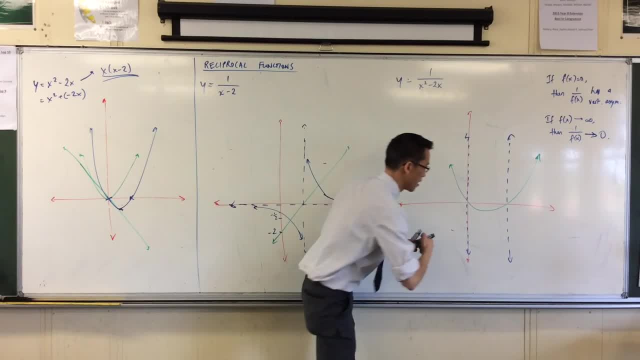 I'm just thinking about the component function, by the way, Like I'm actually thinking about what is the coordinates. It's going to be 1 and 1. take away. 2 is negative, 1, right. So that point is 1, negative, 1.. 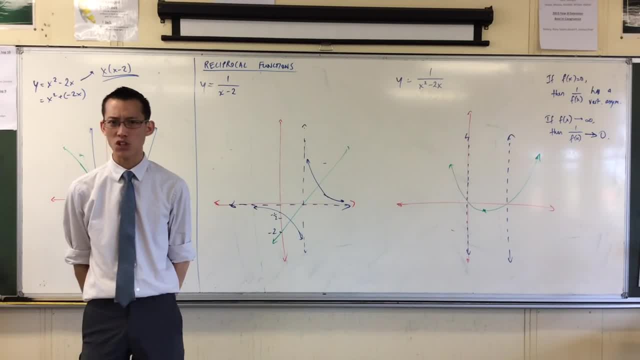 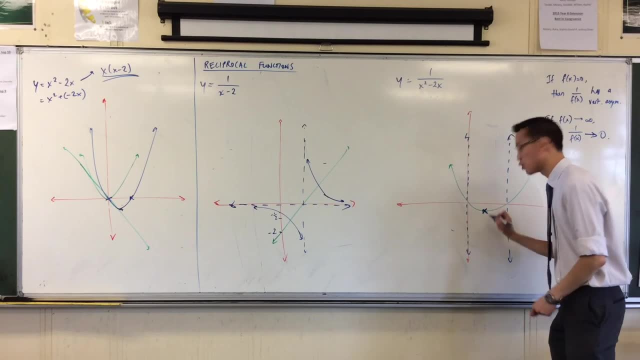 The ordinate is the part I'm interested in. What's the reciprocal of negative 1?? It's negative 1, right. So therefore my actual graph is also going to pass through that point, And that's important to me. 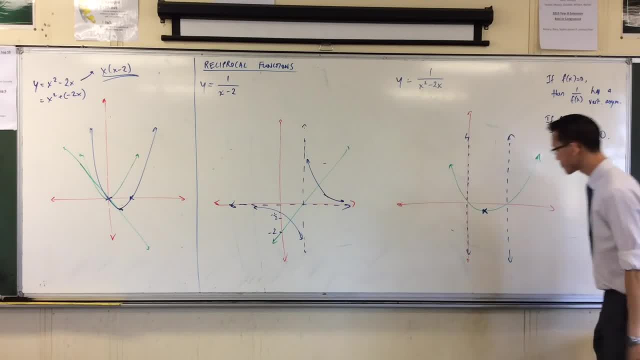 I've said it's there, just like I said this intercept was there, right? Oh, this makes so much sense. Yeah, you can see the behavior. You can understand the behavior now, right, Okay, now let's just look in here. 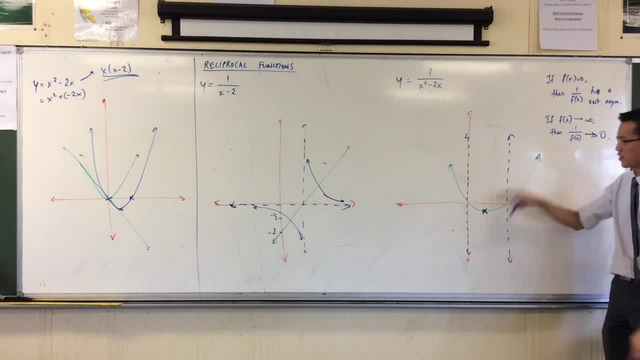 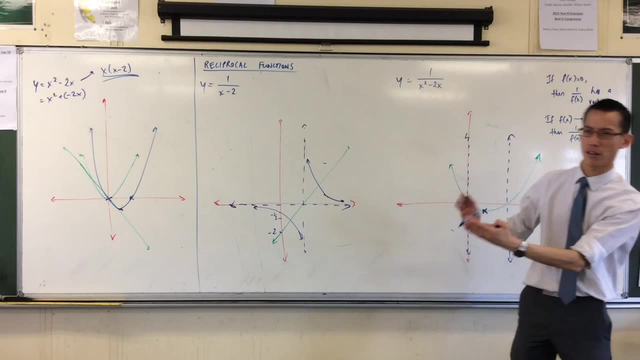 What's happening? Well, I've got, I'm approaching 0, right. So on this side here, my component graph is approaching 0.. So if the components approach 0, what's the reciprocal of that going to approach? 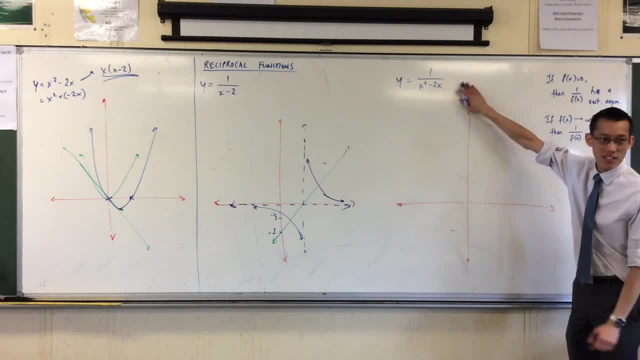 OK, now standard hyperbola. That was a bit boring. If you have a look at something like this guy, you see I've craftily chosen the graph that we just did over there, So let's just draw. here is our component graph. 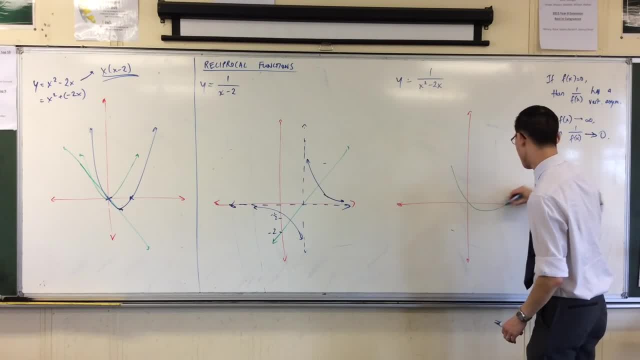 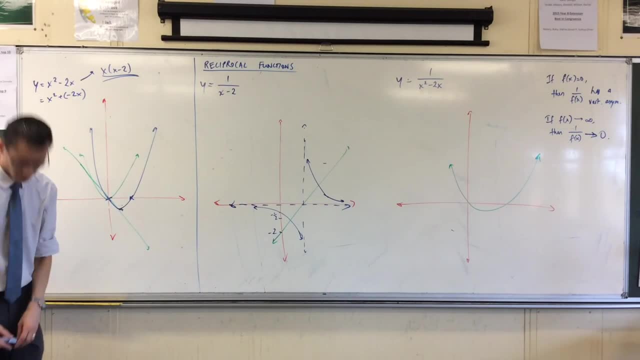 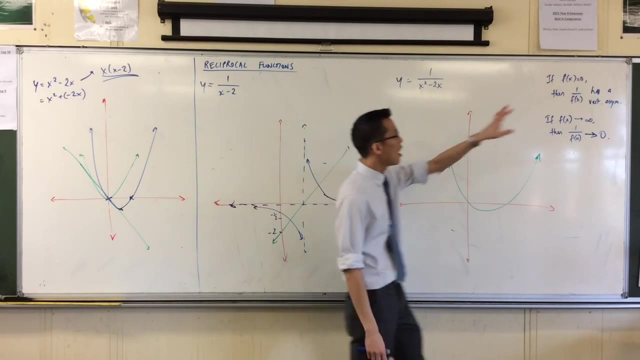 and then we can do our reciprocal. Wait, You already know what x squared minus 2x is. OK, So now I'm going to approach this in the same way. right, I look at the points where my component function is 0,. 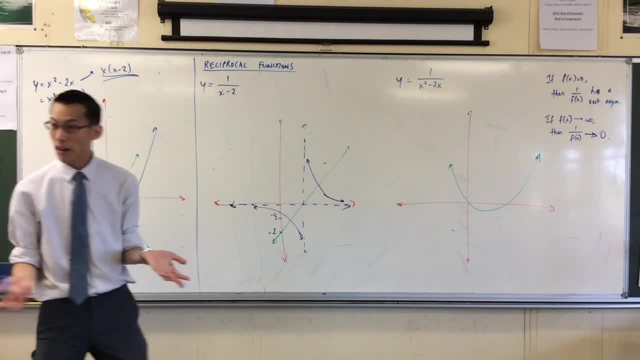 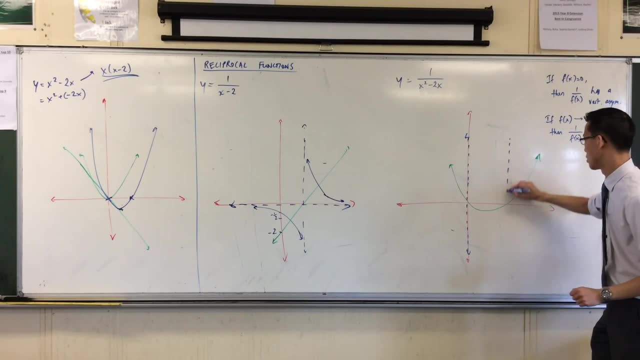 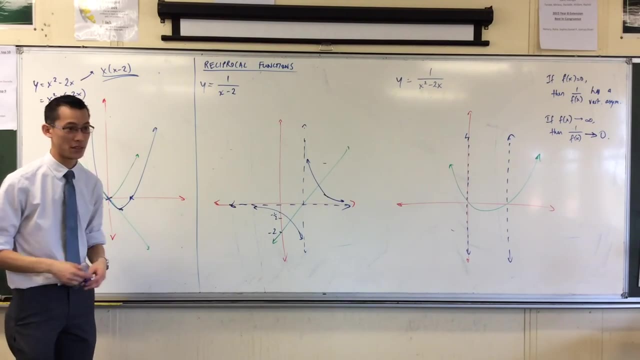 and there are two of them, which means I've got two vertical asymptotes. Let's draw them in. OK, Now again I'm going to look for my important function, My important places, important places. So, for instance, I actually know there's a stationary point here. 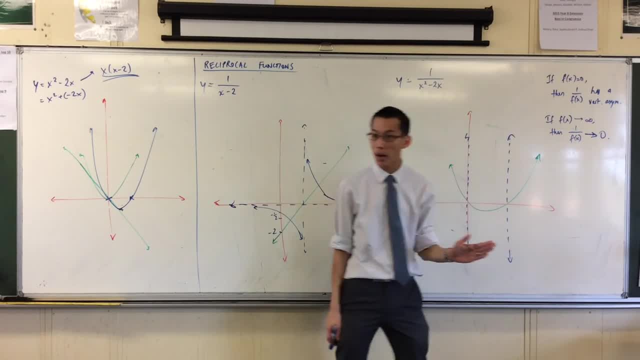 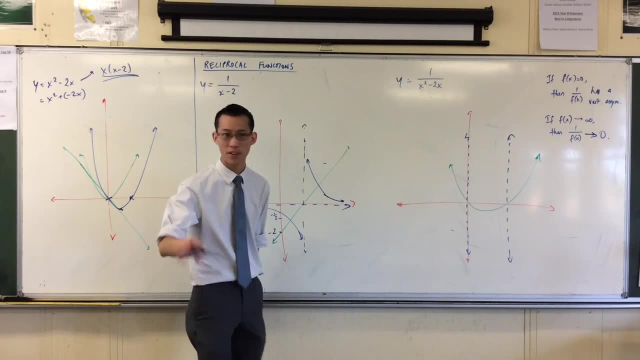 and I can fairly easily work out its value right. The x value is 1.. So what's the y value? What's the ordinate? I'm just thinking about the component function, by the way, Like I'm actually thinking about what is the coordinates. 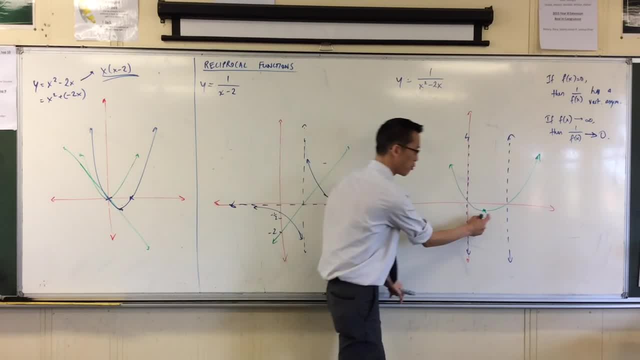 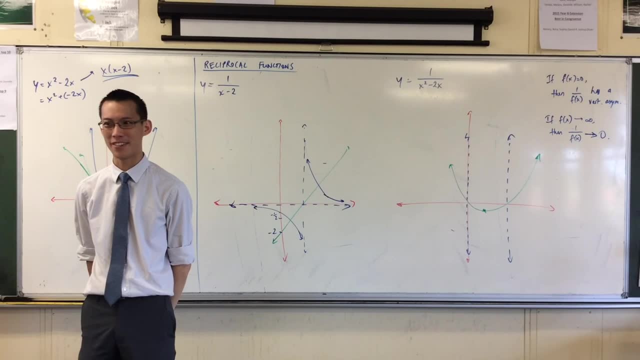 It's going to be 1, and 1. take away 2 is negative, 1, right. So that point is 1, negative 1.. The ordinate is the part I'm interested in. What's the reciprocal of negative 1?? 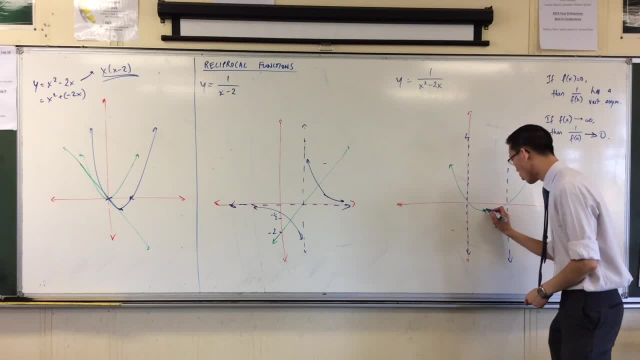 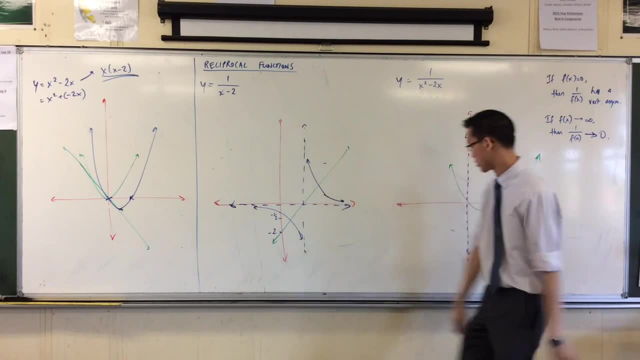 It's negative 1, right. So therefore my actual graph is also going to pass through that point And that's important to me. I've said it's there, Just like I said this intercept was there right. So far, so good. 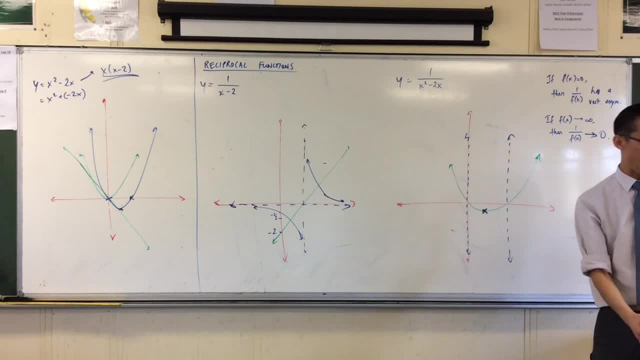 Oh, this makes so much sense. Yeah, you can see the behavior, You can understand the behavior. now, right, OK, Now let's just look in here, right? What's happening? Well, I've got, I've got. no, I don't have this. 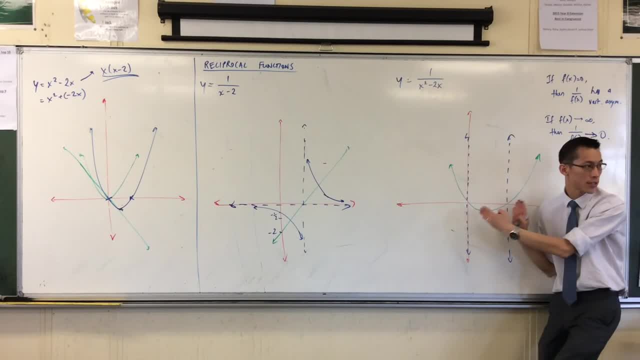 I'm approaching 0, right On each side here, my component function is 0.. The component graph is approaching 0.. So if the components approach 0, what's the reciprocal of that going to approach? Approaching infinity. It's going to approach infinity, right. 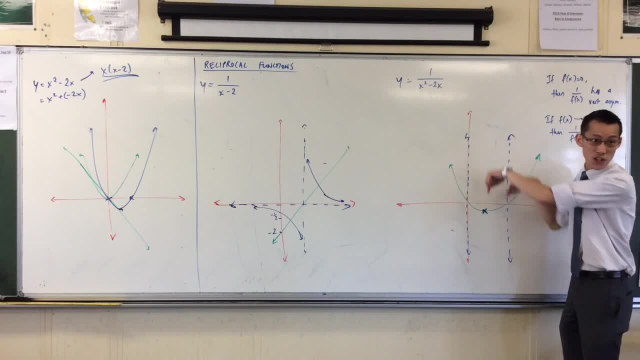 But be careful, I'm negative here. negative, So I'm approaching negative infinity, which, of course, we could have known by drawing regions. But because I'm approaching this in this way, I don't need regions. right, You're going towards negative infinity. so there is my graph. 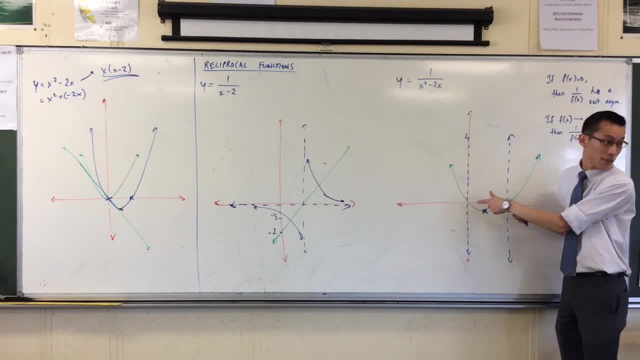 Approaching infinity. It's going to approach infinity, right, But be careful, I'm negative here. So I'm approaching negative infinity, Which of course we could have known by drawing regions, But because I'm approaching this in this way? 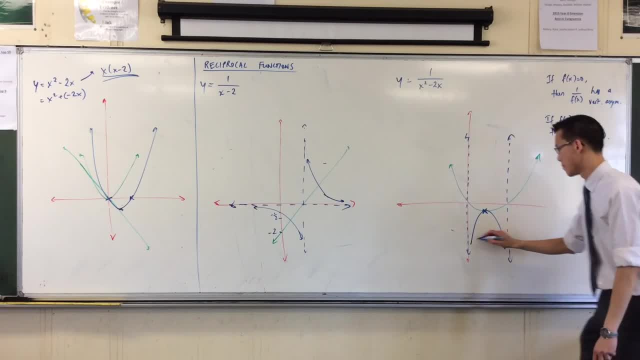 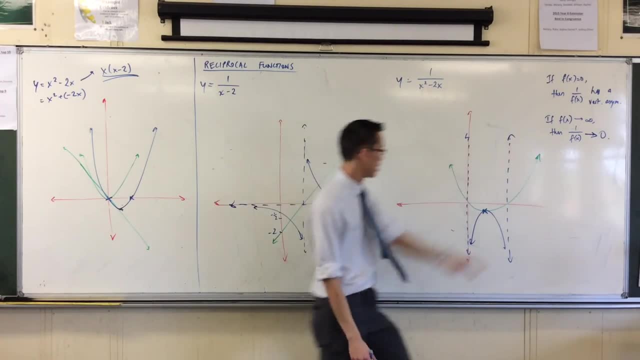 I don't need regions, right? You're going towards negative infinity. so there is my graph Now on the outsides of those regions. I could use the same argument here and here. right, These graphs up here are going towards positive infinity. 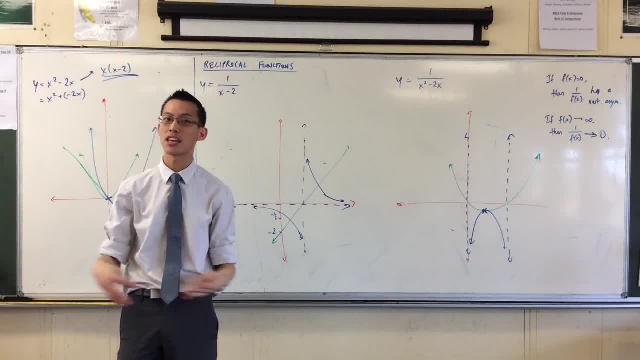 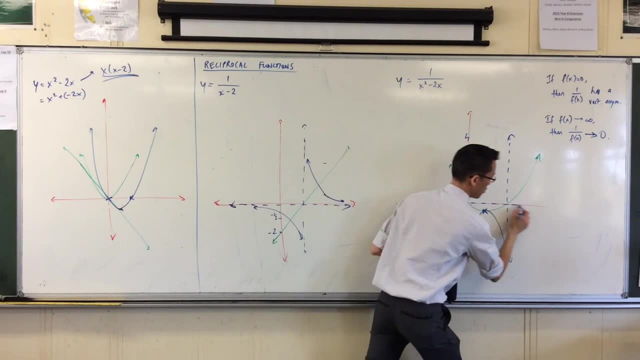 and there's no boundary on those. They're just going to go forever, okay. So therefore, when you take the reciprocal of those, they're going to shrink, They're going to come towards 0.. So that's where my horizontal asymptote. 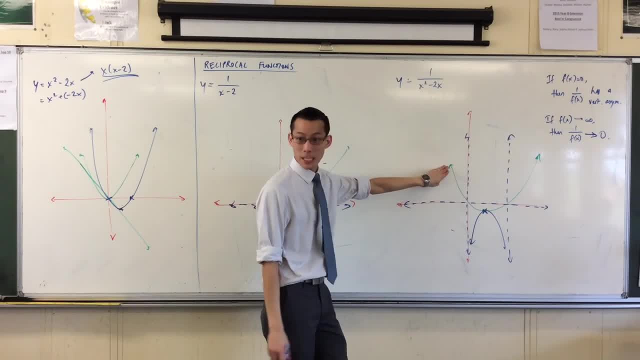 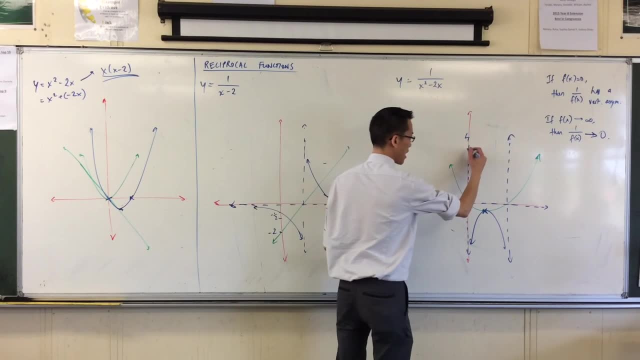 comes from right. You see the denominator. that's my green graph. the denominator is getting huge. So the actual graph, the reciprocal of that, that's how you get these graphs that are going to come down here Now I should really be watching for my points of intersection. 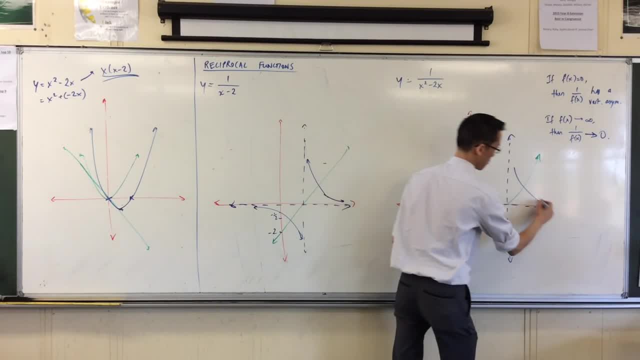 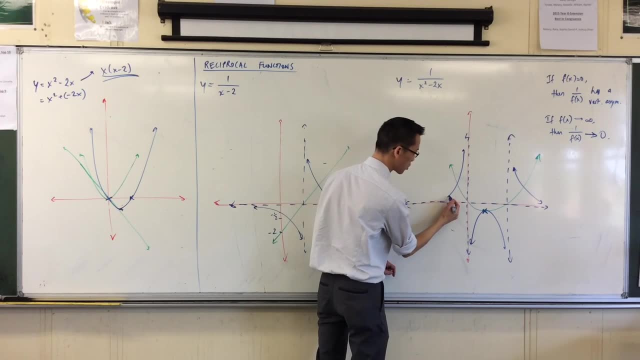 but you can find those. they're not that hard. You're going to get these shapes here, okay, So now you have another analytical tool for well, why do I get this linear shape? And it's like: think about the reciprocals. 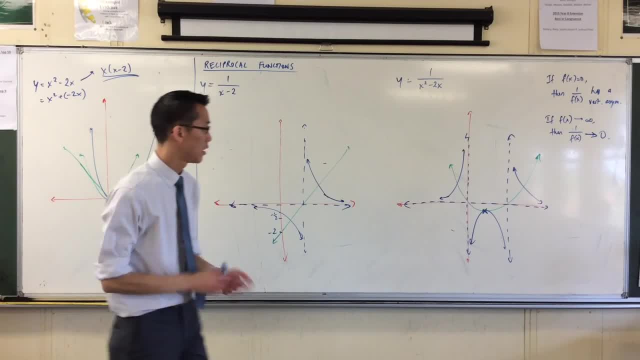 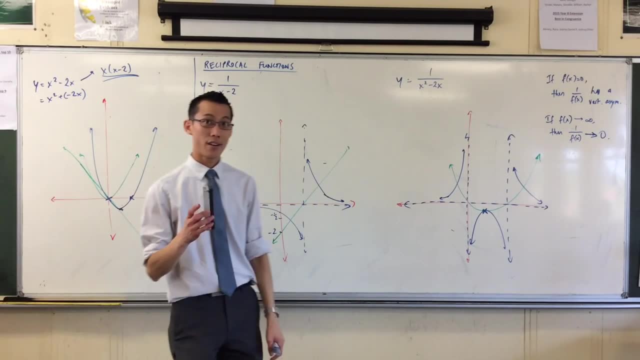 Think about how they're actually forcing themselves to behave. okay, Now one last one. Yep, perfect timing, And we'll do this really quickly. We're going to do cosec x, cosec x, And we're going to think: 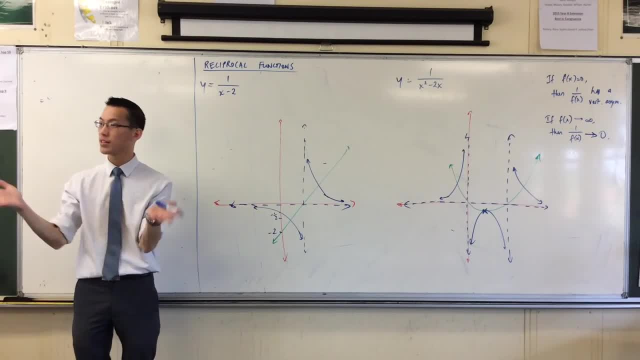 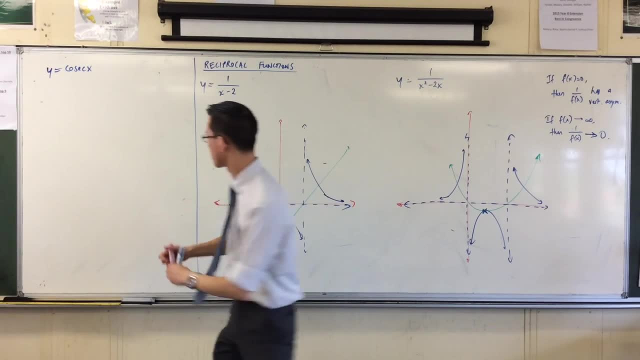 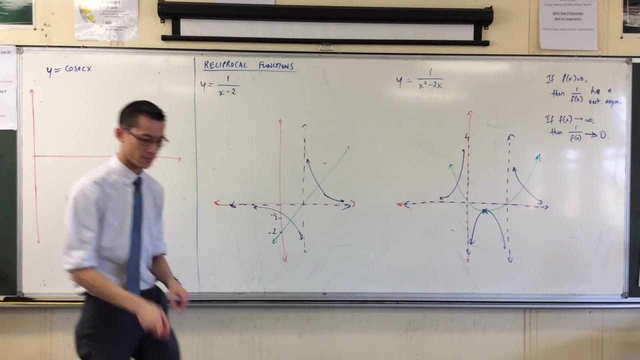 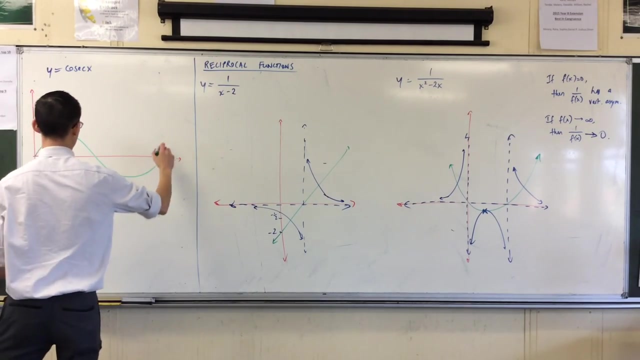 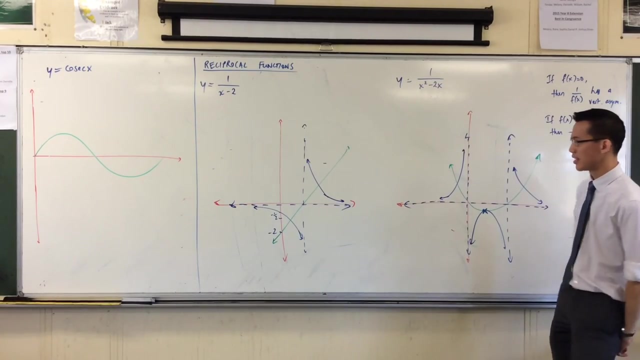 in exactly the same way. Let's draw it from 0 to 360, we'll do 0 to 360.. 0 to 360.. Okay, so really quickly, let's crack through this, because not too much time left right. 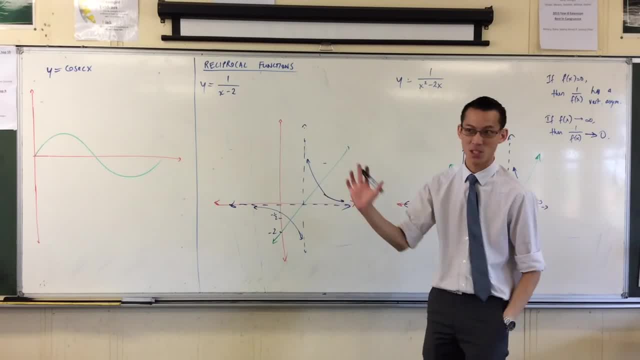 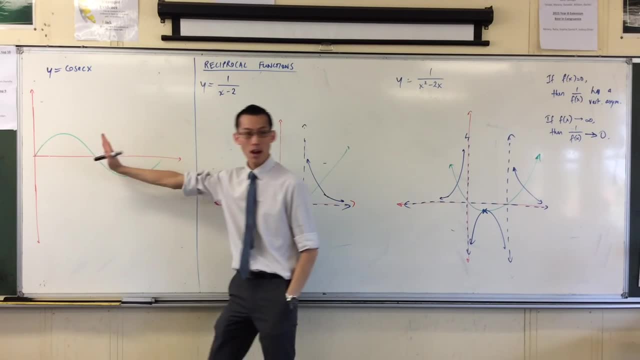 I want to look for important points right Immediately. I see three important points screaming out at me. What are they? I've got zeros, right. I've got roots, I've got x intercepts. So 0 degrees, 180 degrees. 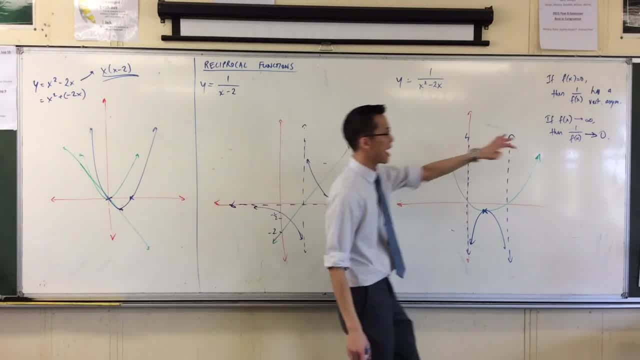 Now on the outsides of those regions, I could use the same argument that I have here And here. right, These graphs up here are going towards positive infinity and there's no boundary on those. They're just going to go forever, OK. 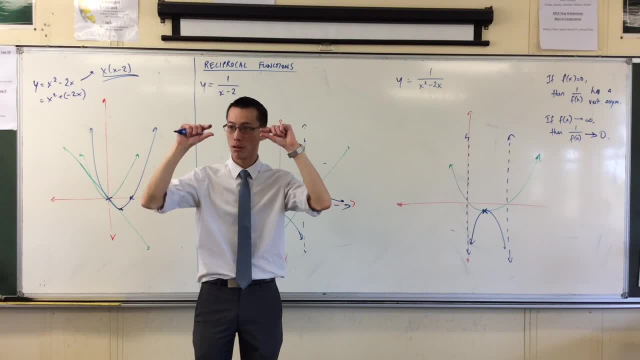 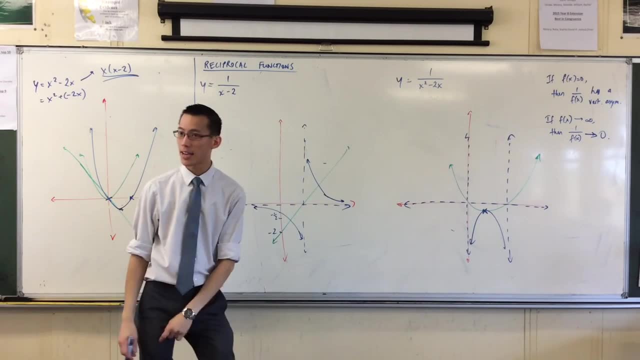 So therefore, when you take the reciprocal of those, they're going to shrink right. They're going to come towards 0.. So that's where my horizontal asymptote comes from right. You see the denominator. that's my green graph. 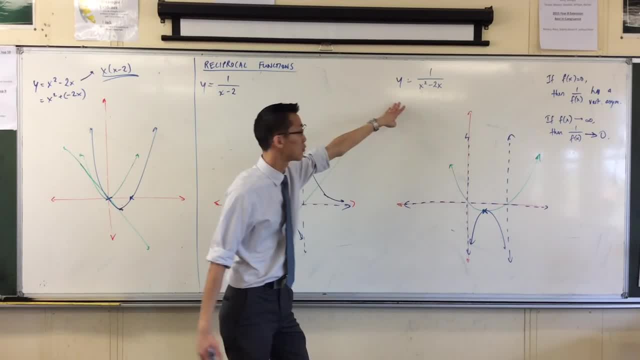 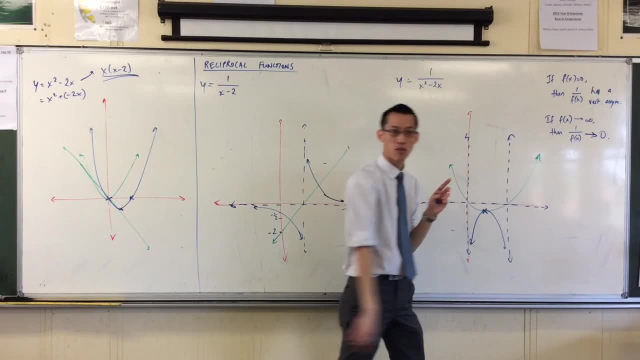 the denominator is getting huge, So the actual graph- the reciprocal of that, is getting small. So that's how you get these graphs that are going to come down here Now. I should really be watchful for my points of intersection, but you can find those. 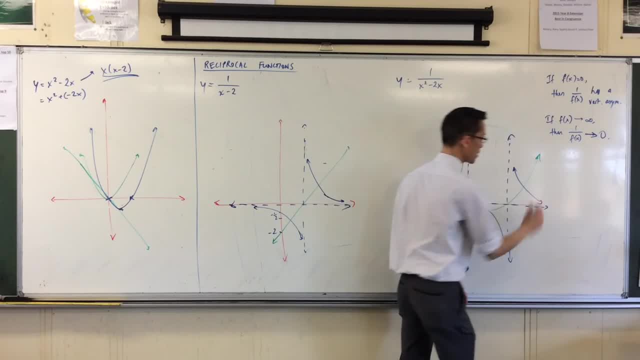 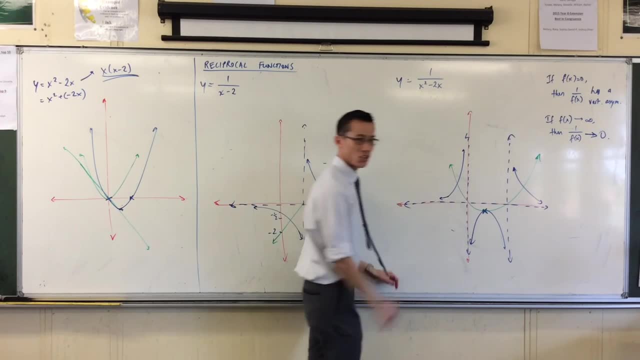 They're not that hard And you're going to get these shapes here. OK, So now you have another analytical tool for well, why do I get this linear shape? And it's like: think about the reciprocals, Think about how they're actually forcing themselves to behave. 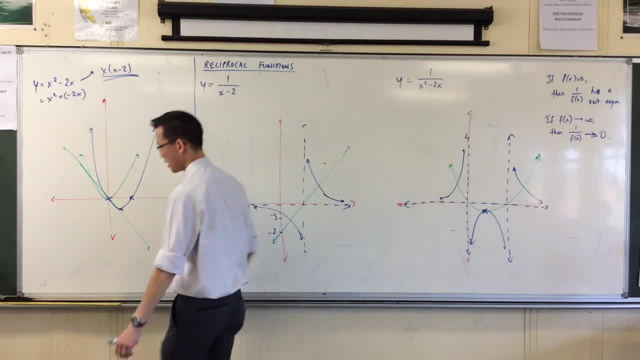 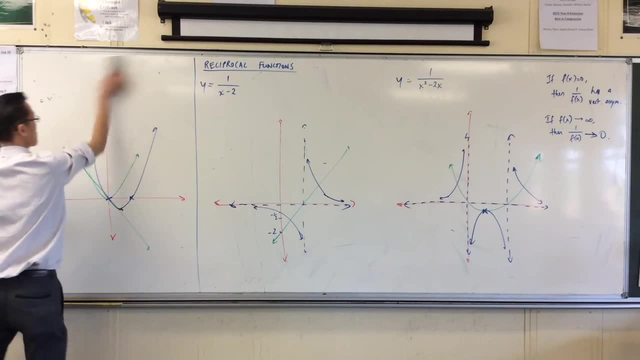 Now one last one. Yep, perfect timing, And we'll do this really quickly. We're going to do cosec x And we're going to think in exactly the same way. Let's draw it from 0 to 360, we'll do. 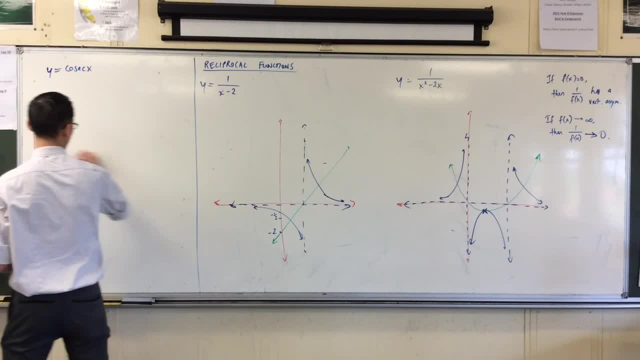 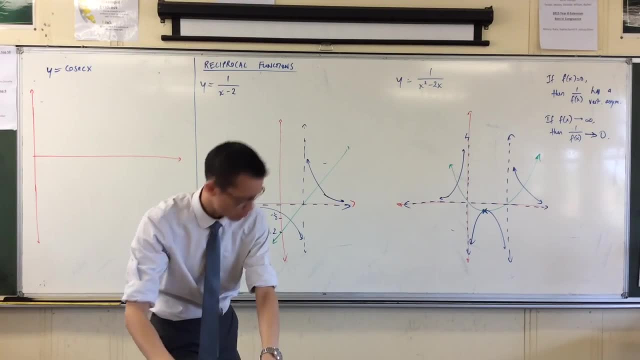 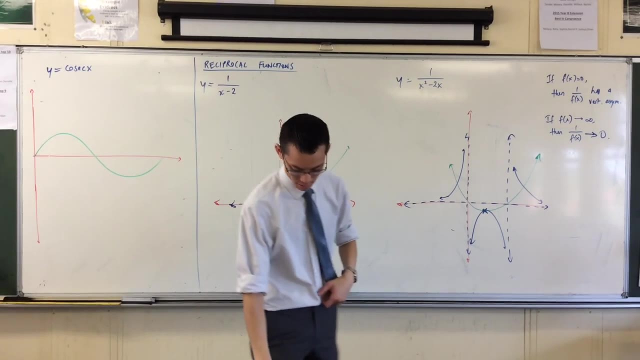 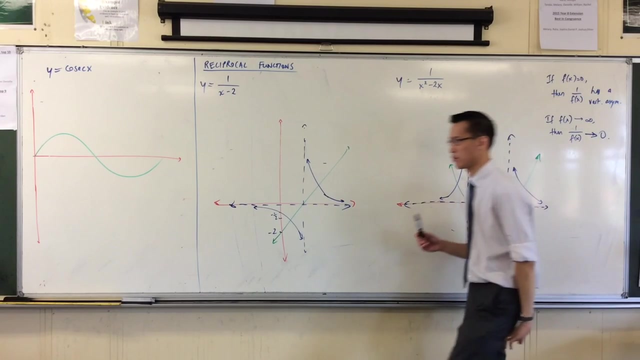 0 to 360.. OK, so really quickly, let's crack through this, because not too much time left. right, I want to look for important points right Immediately. I see three important points screaming out at me. What are they? 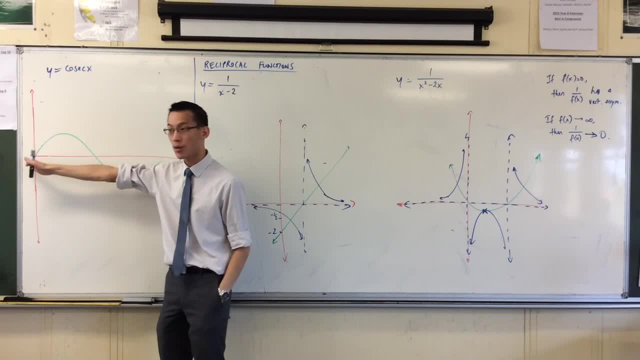 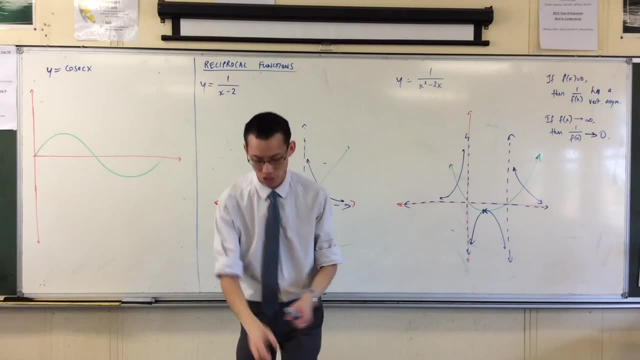 I've got 0's right, I've got roots, I've got x intercepts. So, 0 degrees, 180 degrees, 360 degrees, The function y equals sine x, which is actually what I'm envisaging here. 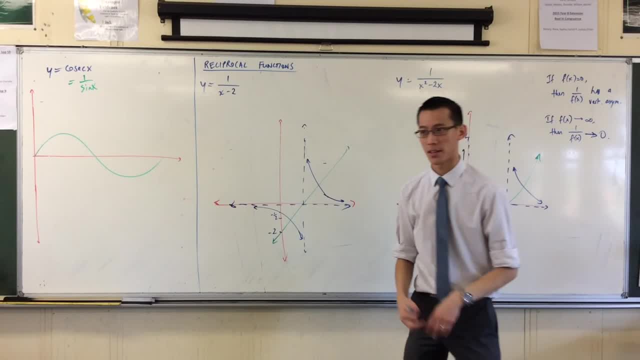 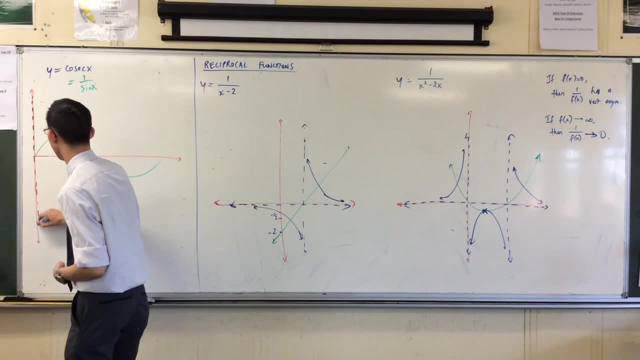 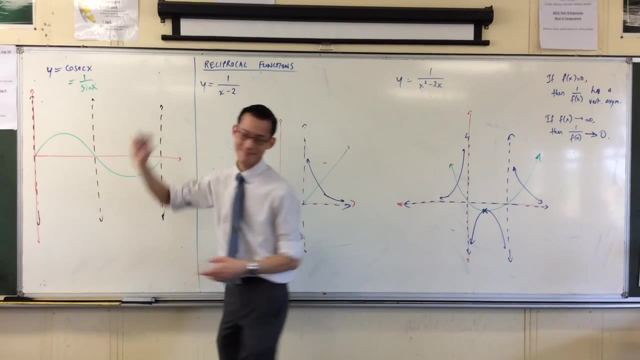 Right Sine x is 0 at all of those points. So that means when I take the reciprocal, I'm getting those vertical asymptotes. yeah, I'm not the only one who's trying to talk over. OK, now I've got those in place.